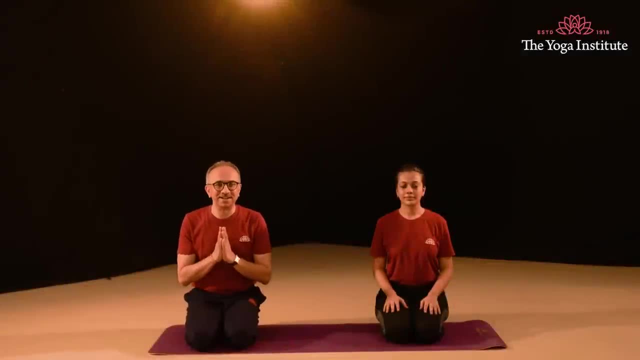 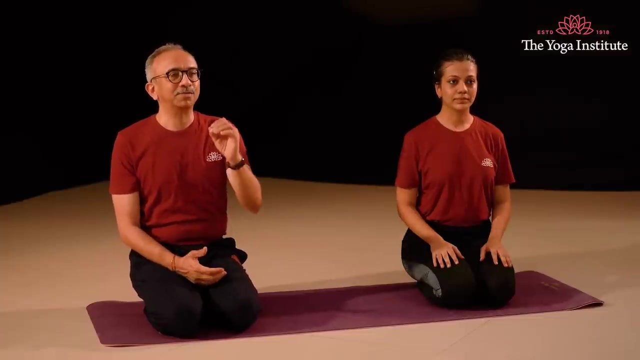 Namaste, my name is Dharmesh Sukhadiya and she is Virtisha, and today we are going to learn a technique called Bhujangasana. Bhujanga is a Sanskrit word. Bhujang means cobra, Asana means posture. 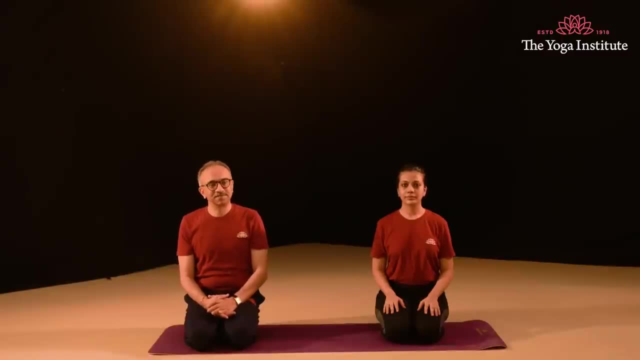 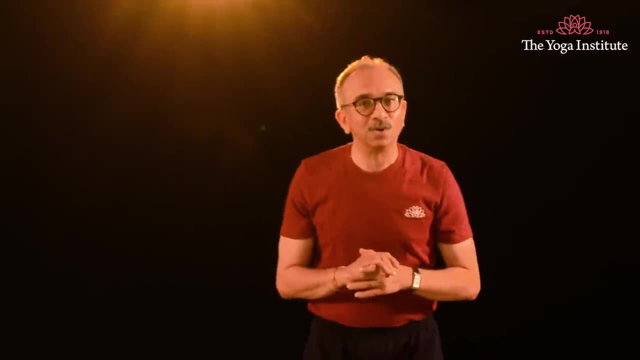 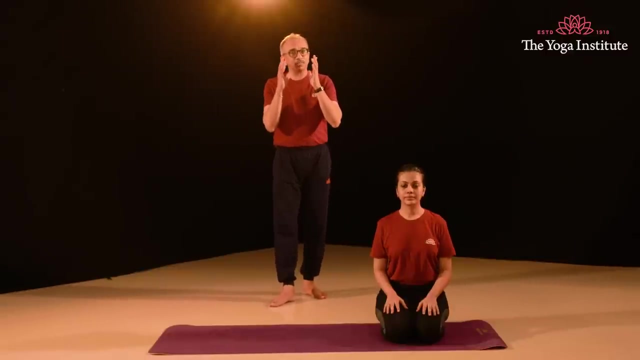 So we will learn in detail about this asana. Let us learn Bhujanga. the requirement of this asana is that one has to lie prone, and this is one of the best backward bending posture in Hatha Yoga. So we will learn this technique. So, Virthi, will you please lie down prone, Turn on the side and then lie down prone. 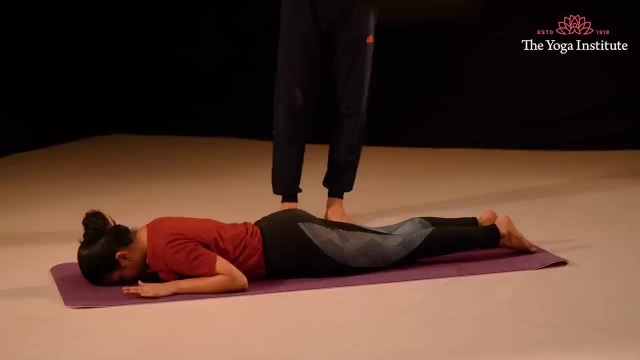 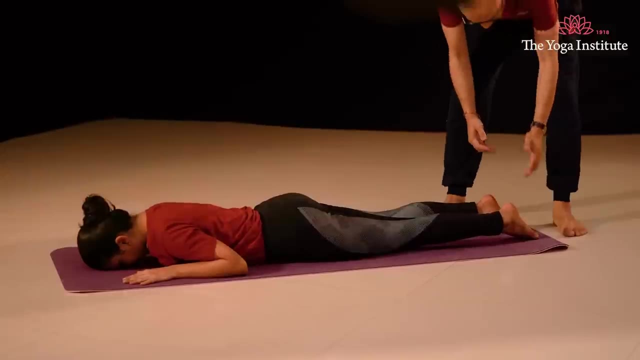 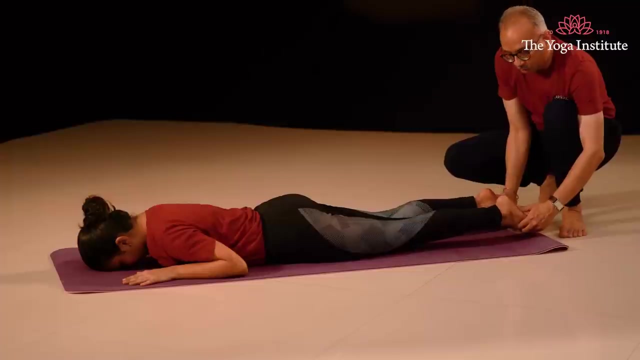 Now, firstly, how people are doing wrong with this posture that I would like to show you. We will start with the legs. first The legs. some people put their legs, their toe, inside. The toe should not be inside. the toe should be out. Both the legs should be together. 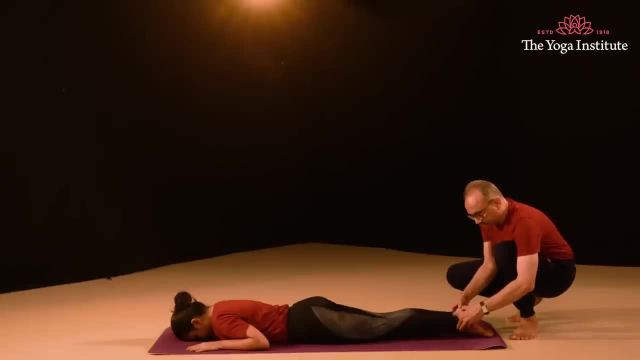 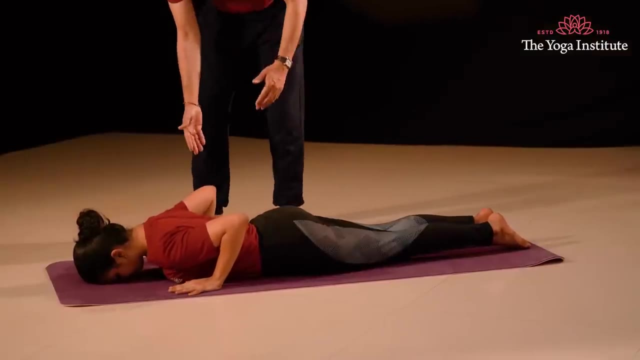 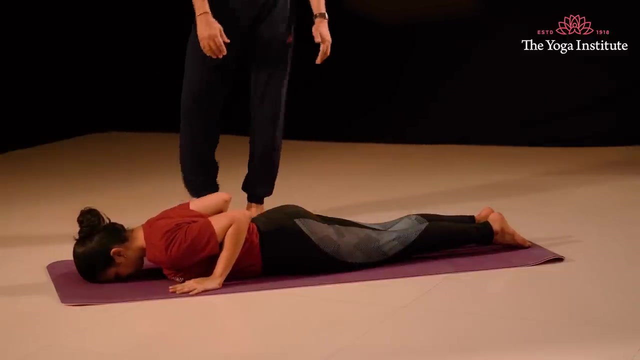 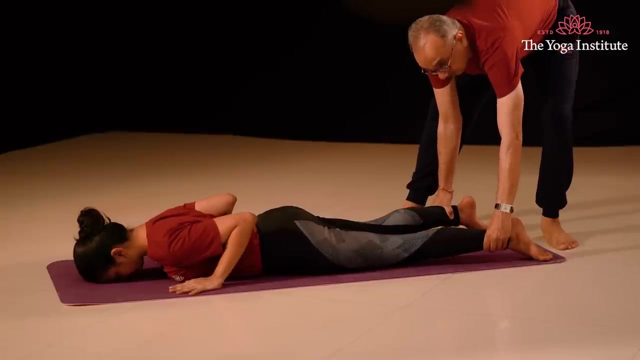 And yes, hands by your chest. The elbow is hugging the body and the forehead is on the ground. Even some people do this technique by taking the legs broad. They do it like this: This is wrong. You should do it both the legs together. 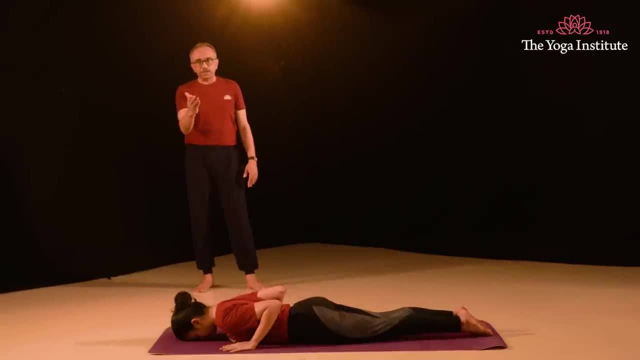 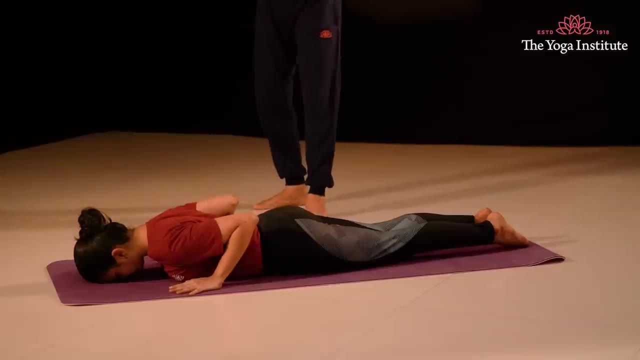 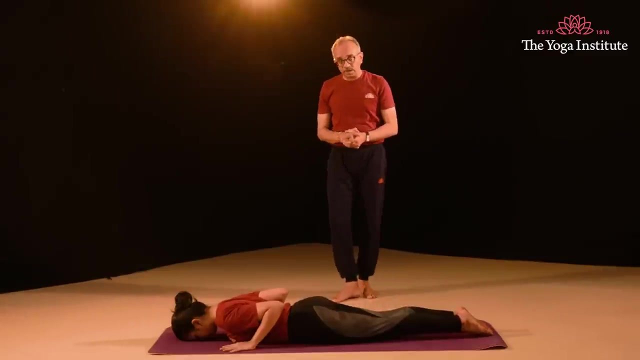 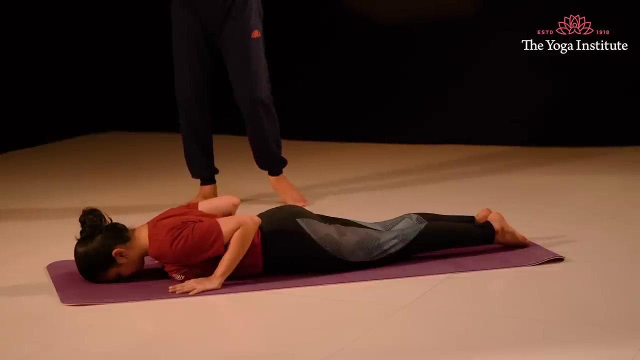 Now there are four main instructions in this particular posture. The first is forehead on the ground, hands by your chest, elbow hugging body and both the legs together. This is very important. Another thing: when you are coming up, you will come up with the strength of your thorax, not the strength of your arms. 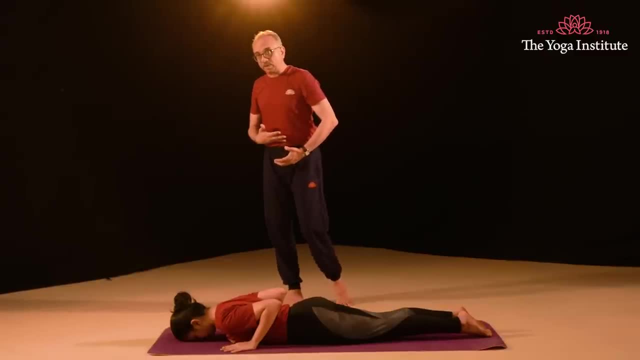 And that too will come up till our navel. only We will not go beyond navel, Because, as you will come up till navel slowly and gradually when you will come up, you will not go beyond navel Slowly and gradually. when you will come up till navel slowly and gradually when you will come up, you will not go beyond navel. 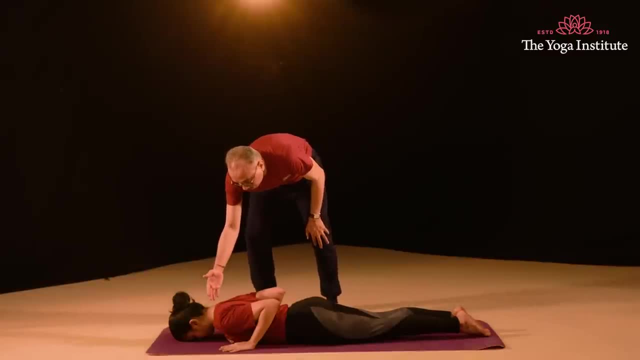 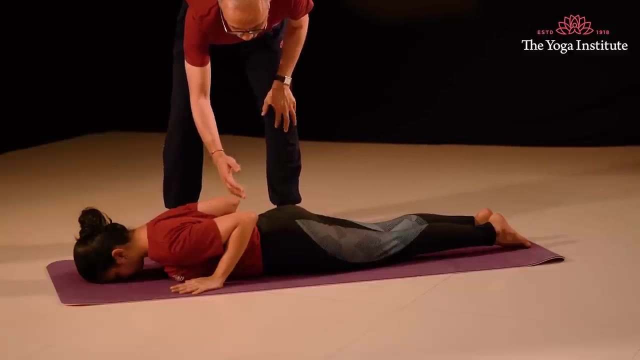 Slowly and gradually when you will come up. you will not go beyond navel. You will come up with first with cervical, then slowly thorax, then slowly lumbar and then slowly the stretch will come to your sacral region also. 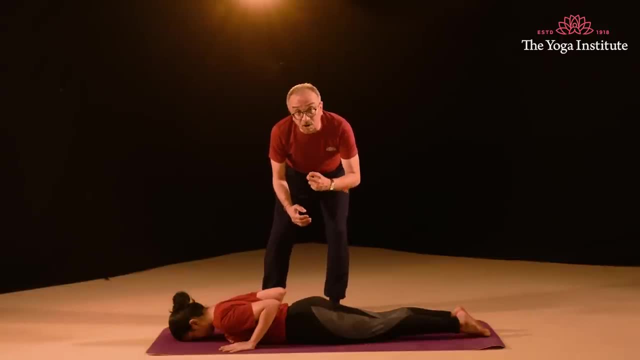 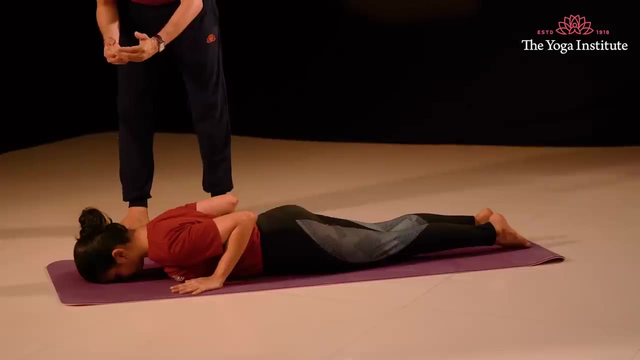 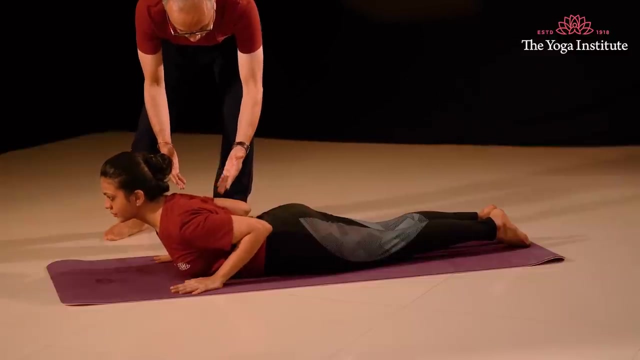 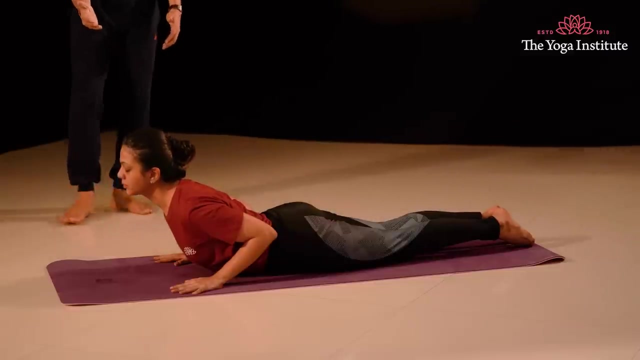 And if you do it perfectly, it will come till your coccyx. So we will do this technique now, Slowly, she will raise her neck Slowly, very slowly. cervical very slowly come up, thoracic very slowly, she will come up till navel, so lumbar region, and she will hold her breath here. 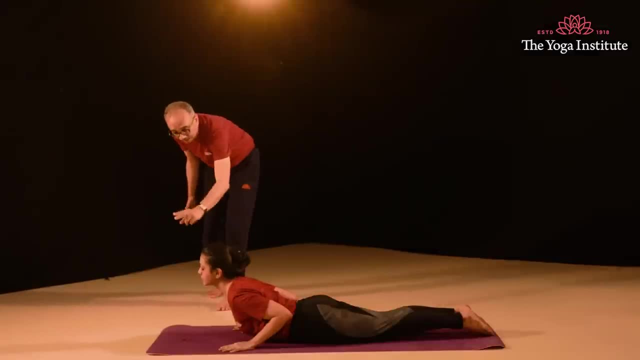 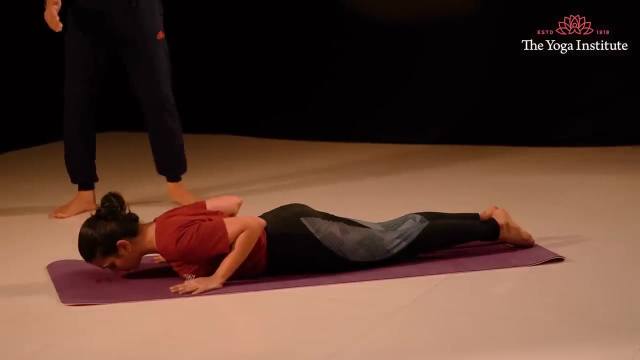 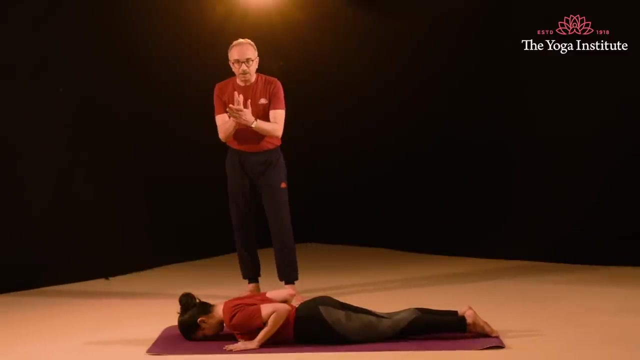 and then the drishti is at nasikagri drishti and then exhaling, she will go down. we will do it one more time with counts. so we are going to do this technique with inhalation- three count, hold for six count and exhaling- three count. see how she is raising. 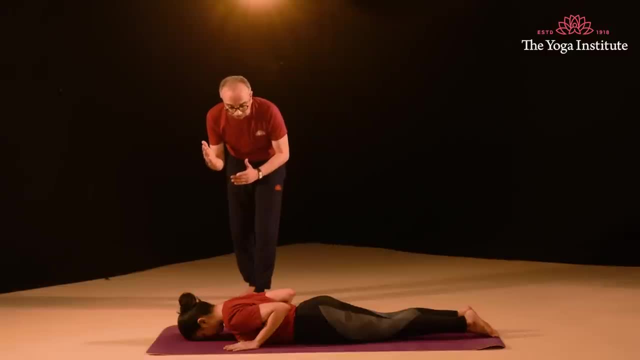 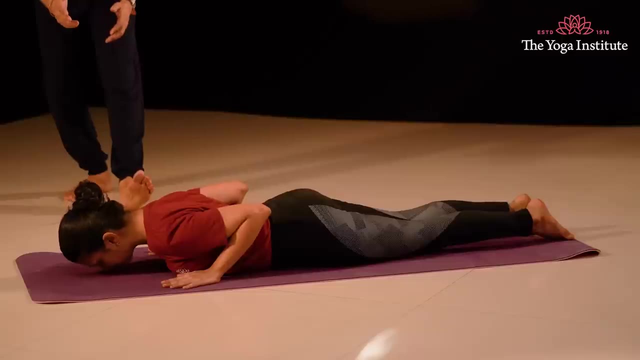 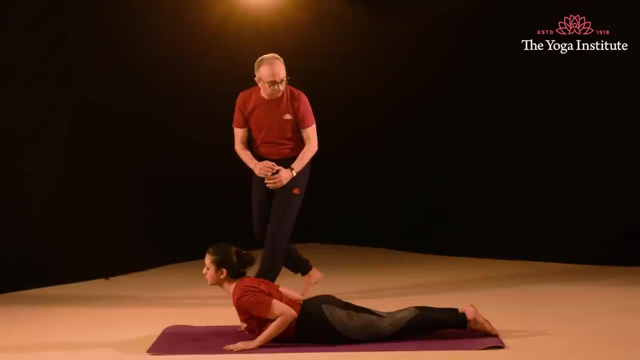 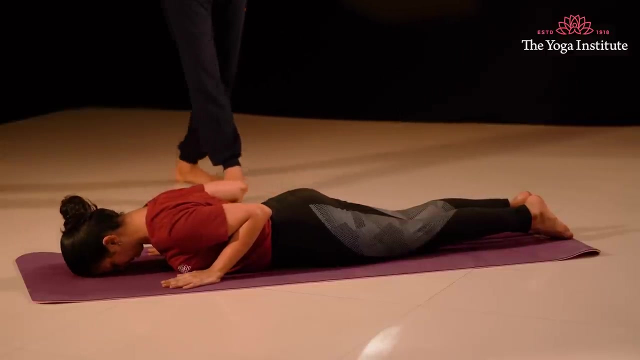 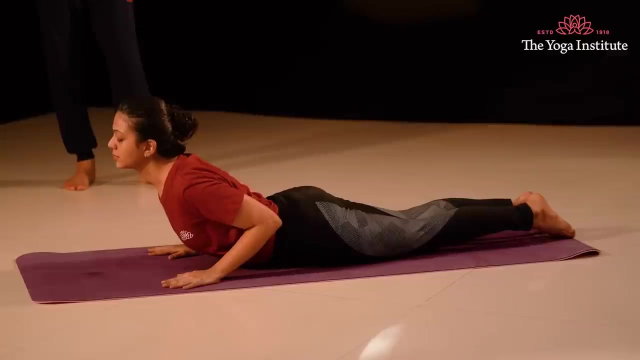 her neck and how she is raising her trunk till her navel. she will raise, so please observe it very carefully. inhale one, two, three, hold your breath. two, three, four, five, six. exhale one, two, three, one more time. inhale one, two, three, hold two, three, four, five, six. exhale one, two. 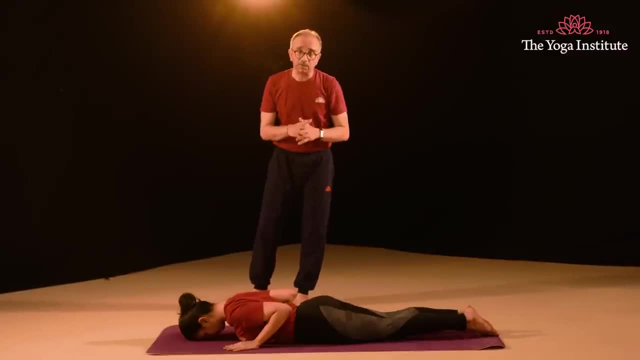 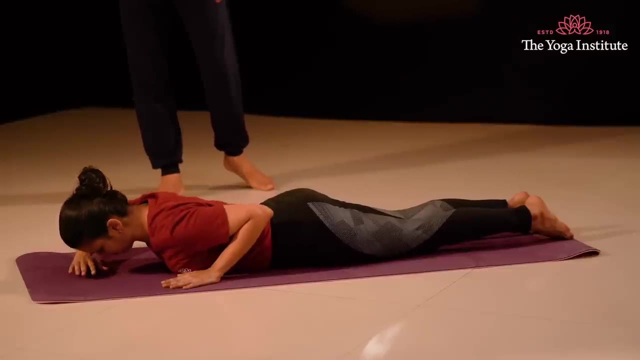 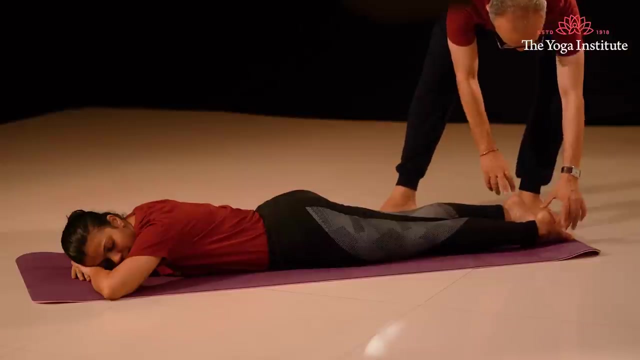 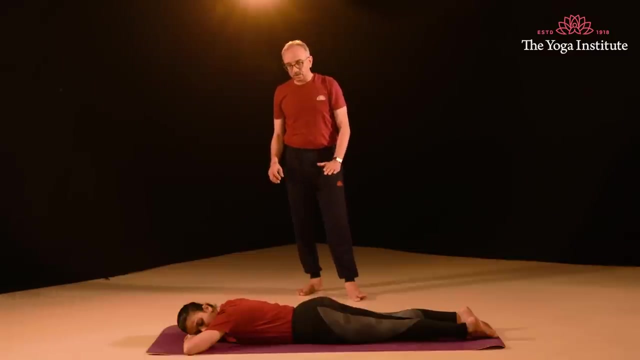 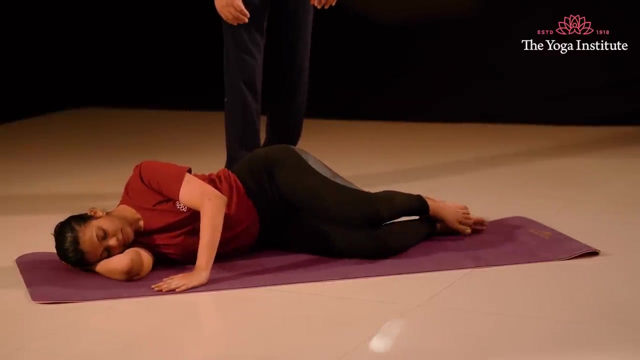 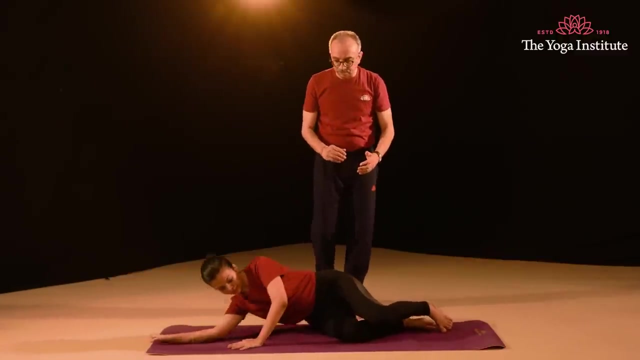 three such six rounds. we have to do it with three inhale, six, hold, three, exhale. after doing that, do the makarasana relaxing posture and toes together, legs apart, normal breathing, very slowly. turn on one side. turn on one side, fold your legs, go into dradasana, take support and sit in sukhasana. 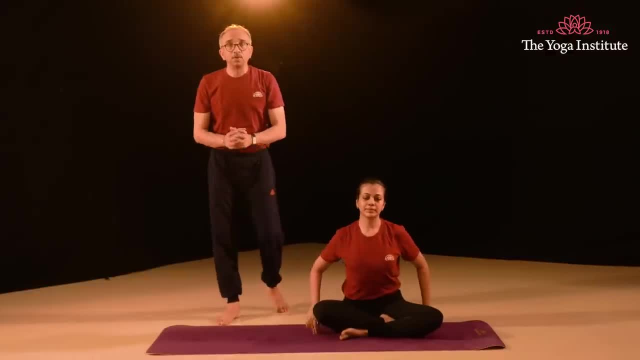 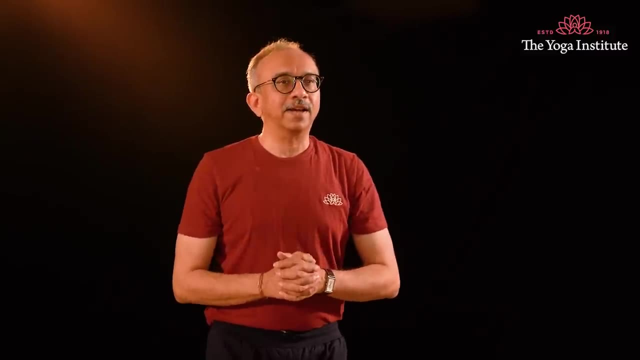 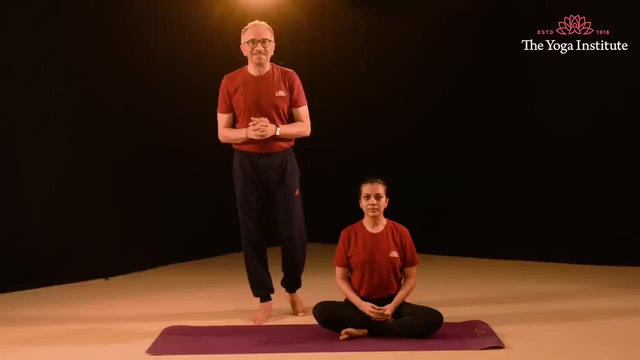 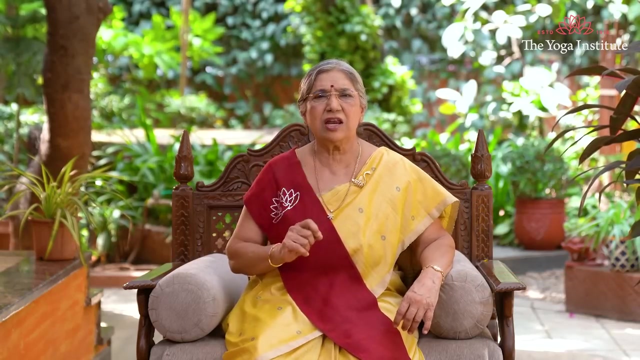 so this was bujangasana cobra posture. so, friends, we have learned this technique and now our guru, hansaji, will throw more light and give more insight into this asana. thank you very much. namaskar bujagasan is a very powerful back bending asana, practicing two to three rounds of this.